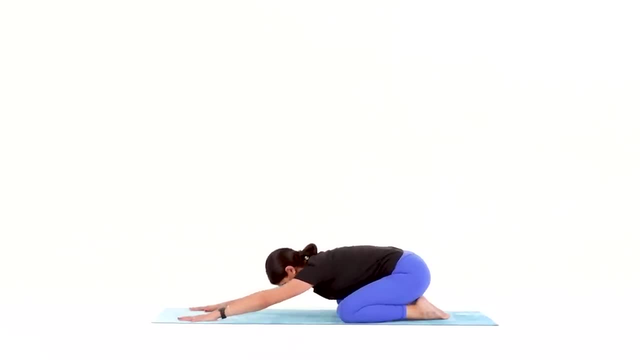 Sit your hips back, Walk your hands forward, Rest your forehead down onto your mat or on stacked fists And feel your breath as it creates space in your lower back. The secret to strength is the ability to hold yourself up when gravity is pulling you down. 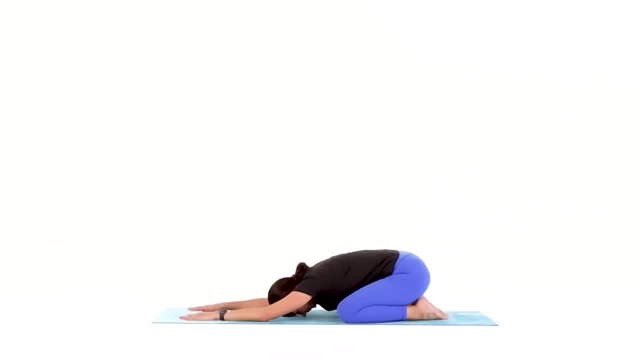 And it doesn't matter if you modified or made it easier or you took a break. You showed up And you held yourself up, even as gravity pulled you down. So take a big breath in, Big breath out, And continue to breathe in and out through your nose and rise up into a tabletop on your hands. 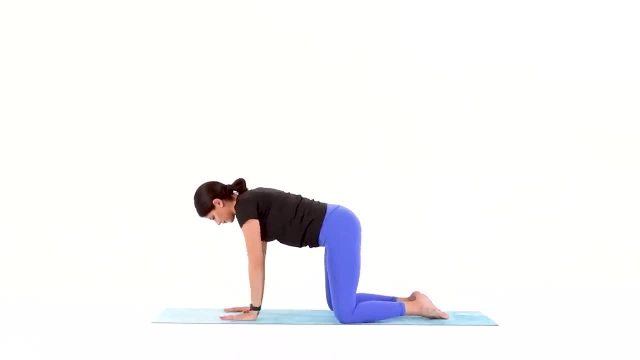 and knees And set it up. Knees directly underneath your hips, Yogi hands directly underneath your shoulders. Firm up your core By pulling your navel in, then hold it there. Then straighten your right leg back behind you Leg in line with your spine, Drive back through your heel And add on by reaching your left arm. 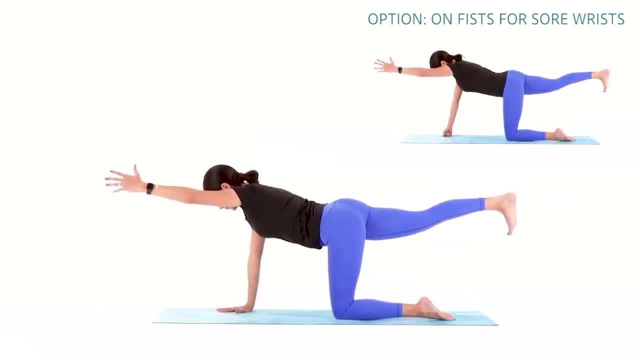 straight ahead of you. Keep your core firm. in between, Breath is calm. Three, two, one Lower back down And switch sides. Extend your left heel straight back behind you, Leg in line with your spine. Keep your navel pulling in And add on by straightening your right arm out in front. 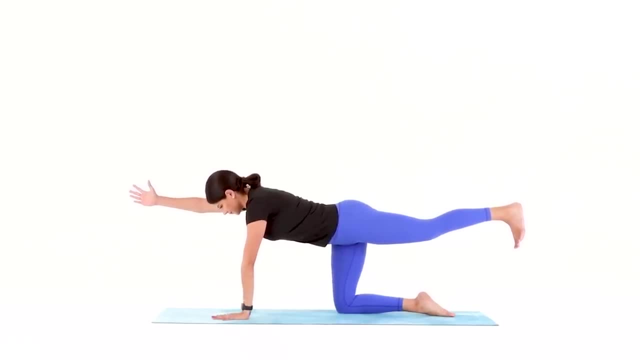 of you And hold: Breathe Three, two, one. Come back to tabletop. Breathe Three, two, one. Come back to tabletop. Breathe Three, two, one. Come back to tabletop. 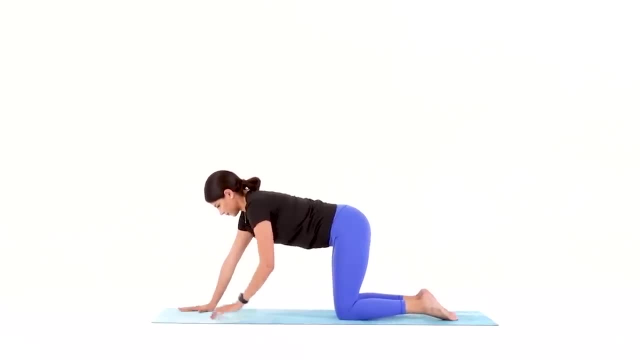 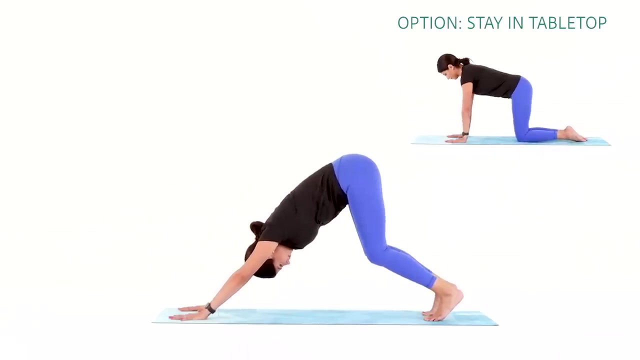 Now walk your hands forward one hand's distance, Then curl your toes under behind you And keep your knees bent as you lift your hips up towards the ceiling For downward facing dog. And to make this down dog a little bit more accessible, take your feet wider, towards the edges of your mat And with a soft bend in your knees. 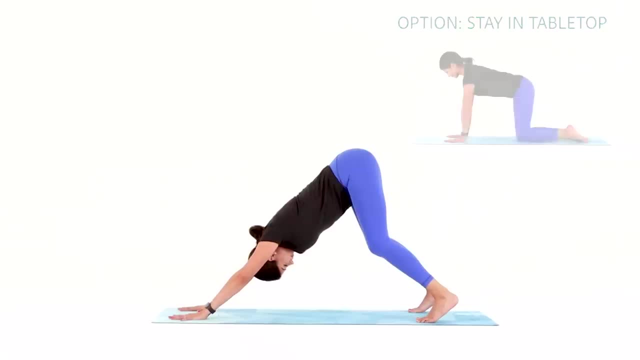 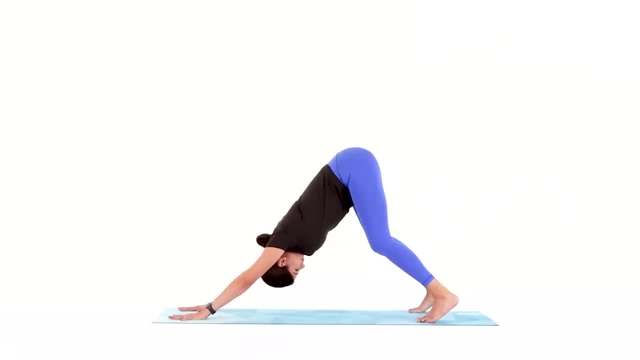 can also do this with your feet. This exercise is intense the first couple of times you practice it, So don't forget to breathe. Then slowly walk your feet in towards the center of your mat, Walk your hands back, then find a forward fold with a爴지만의肌肉, with a generous bend in your knee. so 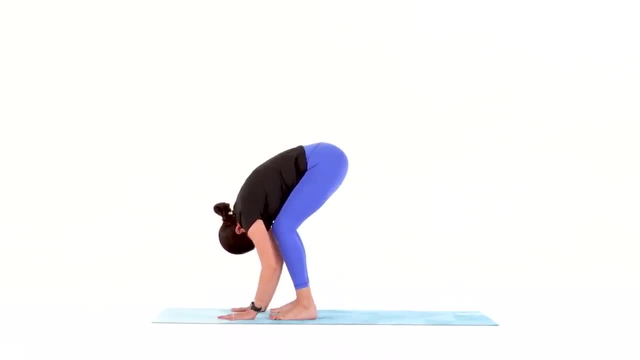 that you can hinge from your hips and fold down towards your mat. You might find a couple of blocks underneath your hands. are very healthy to bend. They are hurting your hips, Maybe helpful to help support the weight of your upper body. but if you use blocks or not, I really want. 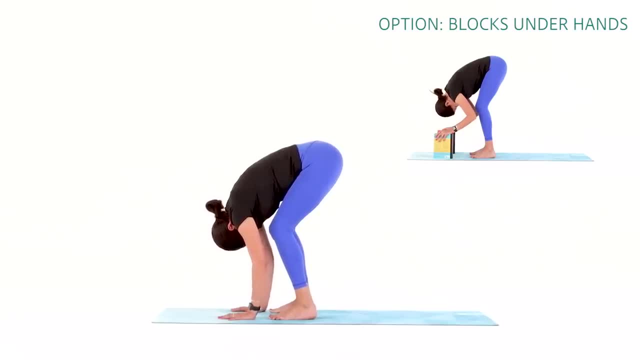 you to focus on folding your spine down towards your mat, relax. your neck. head hangs heavy and if you want to add on here, you can add ragdoll arms by crossing your arms, hands at your elbows, swaying a little bit side to side, and feel your breath travel up and down your spine. now release your. 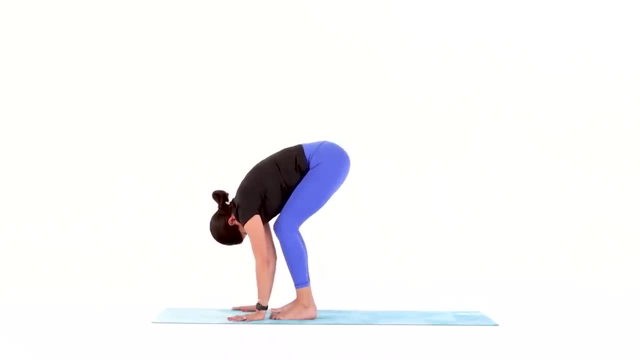 ragdoll arms or move your props off to the sides and take your hands to your thighs, right above your knees, for a halfway lift. so, with your hands on your thighs, push your chest forward, finding a flat back. lifting up halfway now. the flat back here means that I want you to get that plank. 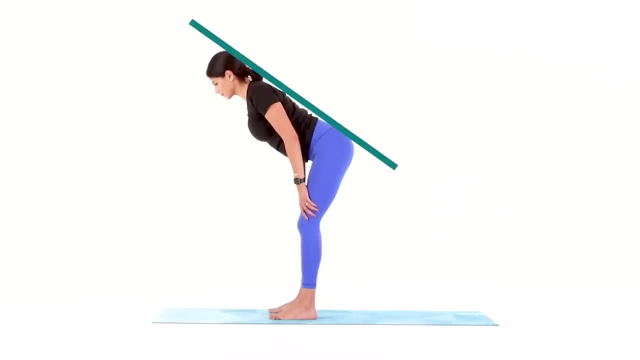 flat back from your hips to your shoulders, to the back of your head. so pinch your shoulder blades together behind you, lift the back of your head up and even with a soft bend in your knees, you'll find that if your hamstrings are tighter, the angle of your flat back is higher. it's not. 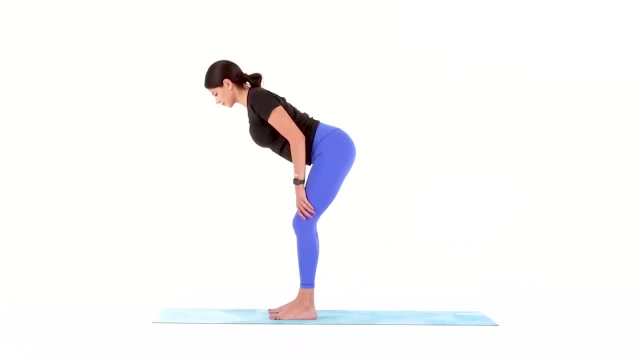 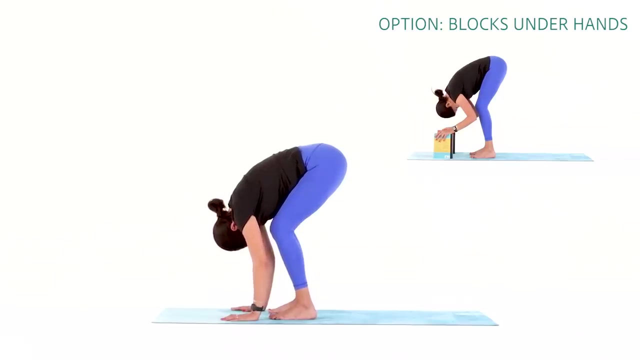 about being parallel to the ground. it's just about finding your flat back and take a big inhale, exhale to forward, fold completely, fold down towards the mat, let your spine round. now let's set up a chair pose. keep your feet where they are, deeply bend your knees, sit back into your hips and 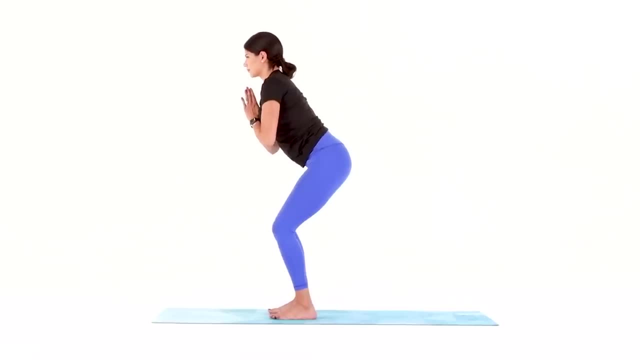 bring your hands together at heart center, sitting back as if someone's scooting a chair in behind you. so you're kind of standing in a half squat and your glutes, your hips, they're probably feeling it. so stay low and relax and take a peek down. you should be able to see your toes past your knees. if not, you need to sit. 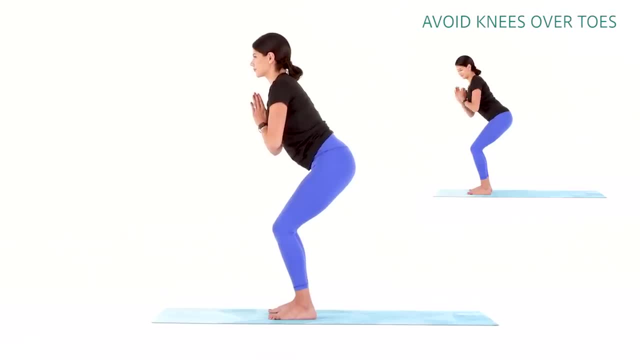 a little bit deeper. you're here for three, breathe two, I know you feel it. one forward fold- wow, that's gotta feel good. to make your folds easier, you can always take your feet a little bit wider, and a generous bend in your knees always helps. next, let's 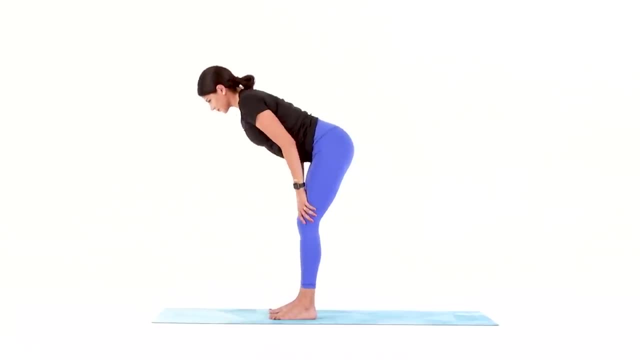 find that halfway, lift again. slide your hands up your shins, place them on your thighs, then press your heart forward. pinch your shoulder blades together behind you and press your chin back, pressing the back of your head up. find the flat back that works for you today, knowing that. 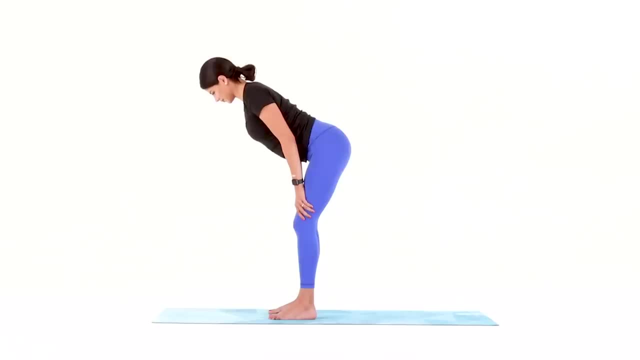 it might not be perfect, that's okay. we call this a yoga practice. take a big inhale, exhale forward, fold, then plant your hands down on your mat and step your feet back into a tabletop on your hands and knees and from your tabletop come forward into a Modified high plank. so a straight line. 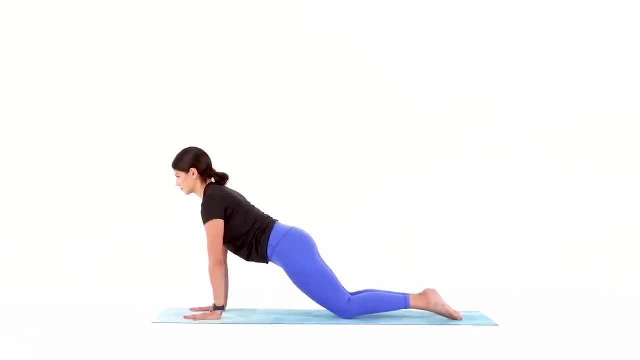 from your knees, through your hips, through your shoulders, through the top of your head. hold yourself here, firm up your core, take a big inhale, inhale to lower your plank down towards the mat, bending your elbows, and pause when your elbows touch your ribs and lower down the rest of your way onto your belly, settling up your lower back on your side, regretting. pulling your heart out and doing half step. shoulder such a great exercise to get that. glutes and gluts warmups much better than the other domes, or coming up a bit lighter. DAMN Gastric Abvention: calm meditation, sitting at the back and released weight after. listen to this. 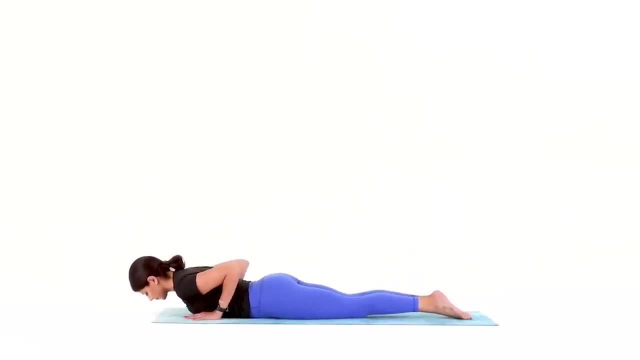 ましょう, back to the acupressure. next, go seated, stand next to a chair, let your foot touch your neck, cooking off that. sit for about 30 seconds. 3 sets rest, which are being relaxed for now. so' your low cobra, zip your legs and feet together to touch top to your feet, press down into your mat. 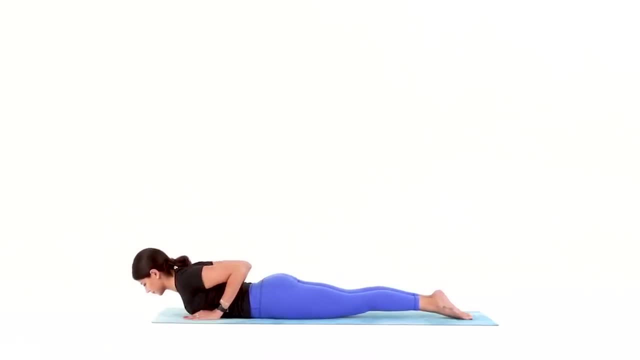 with your hands underneath your shoulders, pinch your elbows together behind you and peel your chest up off the mat using the muscles in your back. so see if you can just prop your hands up on spider hands, just on your fingertips, so you're not using the muscles in. 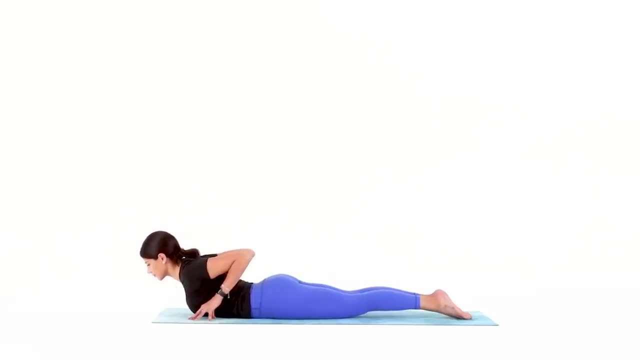 your arms for this low cobra. instead you're using your back. feel yourself bob with your breath. three, two, one. release down to your mat. then take your time as you press into your hands, lifting up into your tabletop and back into an extended child's pose, with your knees wide, shins like a v, big toes. 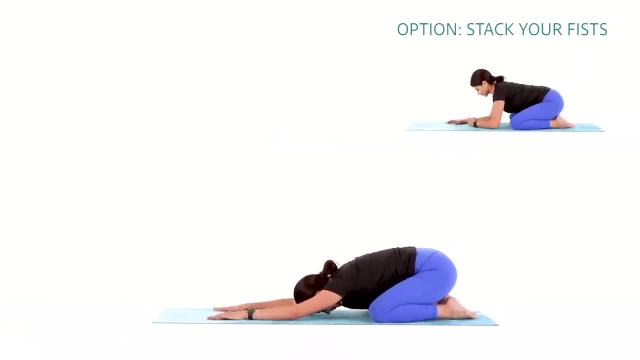 coming together behind you, sit your hips back towards your heels, walk your hands forward and rest your forehead down onto your mat and completely relax deep in your breath, in and out through your nose. that was hard, definitely outside of your comfort zone. i'm sure it was meant to be hard. 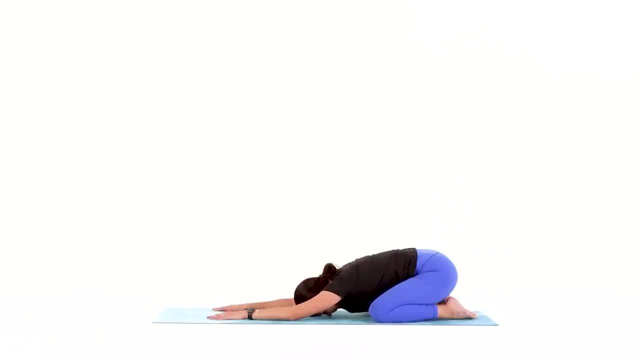 and it was meant to be outside of your comfort zone, because it's through the discomfort that you grow, it's through the challenge that you find your strength. i know it's close to reality from my point of view. keep pushing yourself deep. take a big breath in through your nose. 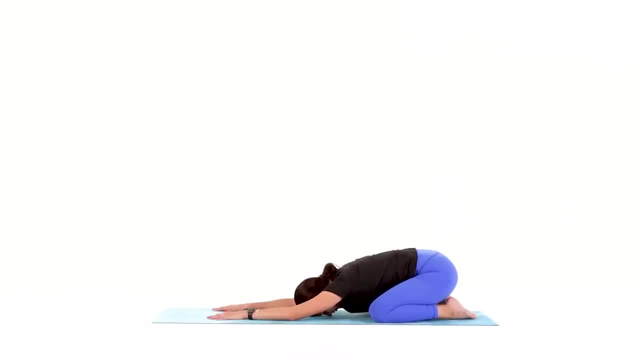 and out through your mouth. so those are some of the случайities that I think we should be being possesed with when we are going into water. as we jumped west in the book, i'm hoping that you definitely will have some of these tips coming your way. 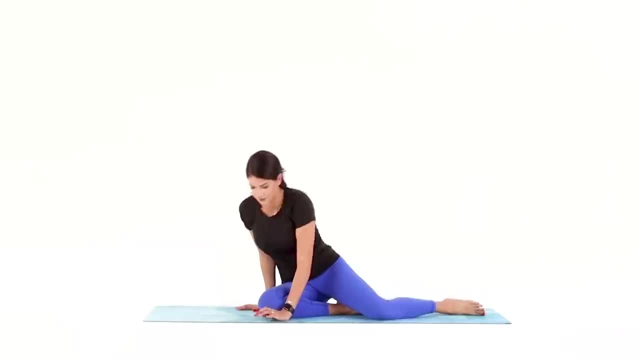 with your challenges, bolstering your breathing, or keep it out into water and continue sitting up tall. when you do that, bring your hands together at heart center. There is a place inside of you where the entire universe dwells. This place is of love, light, truth and peace. When you are in this place,